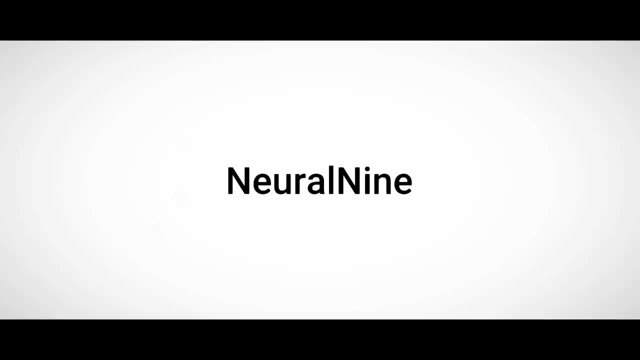 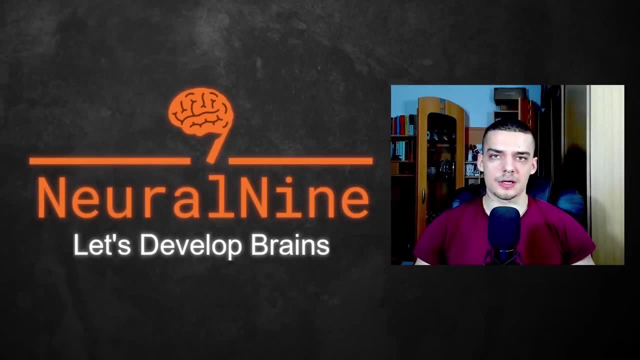 What is going on, guys? Welcome back. And today I'm going to give you a brief introduction into the Seaborn module in Python. And the Seaborn module is a wrapper around Matplotlib, So it uses Matplotlib and it allows you to design to create attractive and good looking statistical 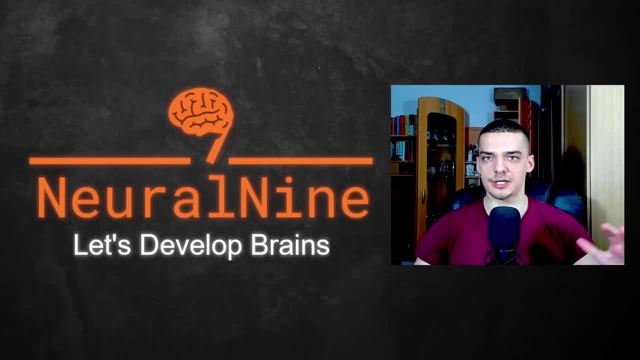 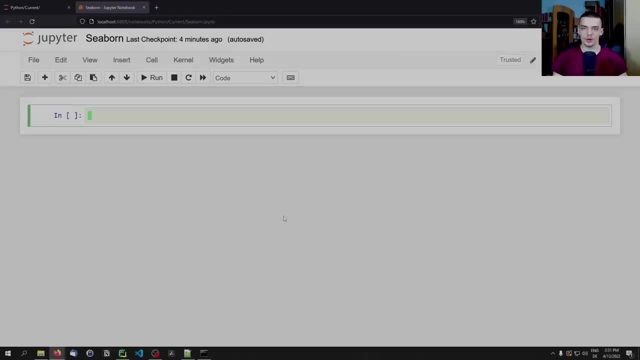 graphs that are quite complex, So it provides a high level interface. it makes it easier for you to create such graphs, And this is what we're going to take a look at today. So let us get right into it. Alright, now, for today's tutorial, I'm going to use an IPython notebook or more. 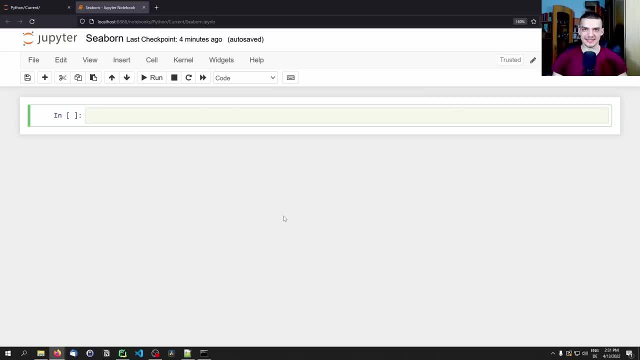 specifically a Jupyter notebook, And I recommend you do so as well, because that allows you to execute individual cells of code, So you don't have to run the whole script when you change something or add something. you can just run individual cells and all the variables, or 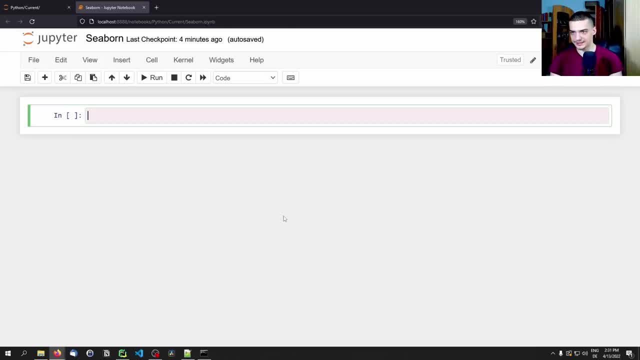 data sets are still stored in the RAM. So let me show you quickly an example here. if I say a equals 10.. Now I'm in a new cell and I could just say print a. and I can go down here and say print a. 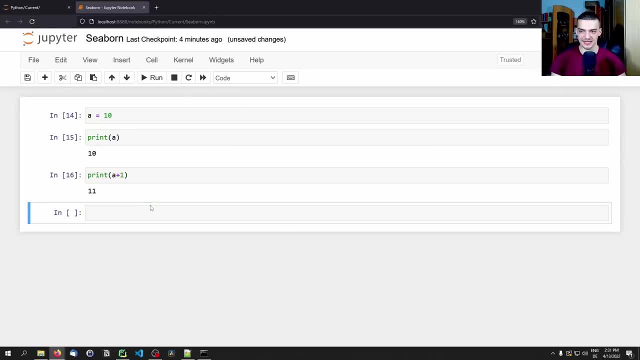 plus one, And I don't have to constantly execute all of the statements that come before, which is particularly useful if we work with data sets and visualizations. So I don't have to look at all the graphs that I have plotted before In order to see the newest graph, and I don't have to delete code. 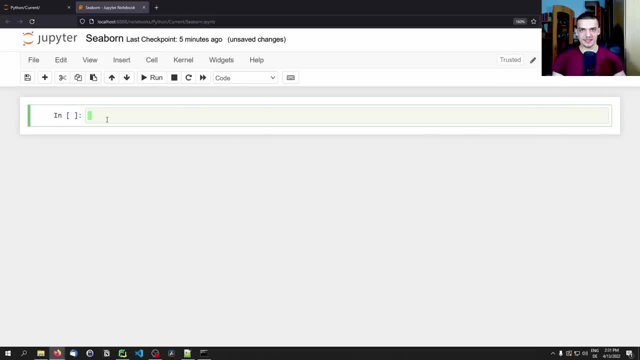 in order to be faster, I can just run individual cells, Which makes a lot of sense when working with data sets. However, if you don't want to use an IPython notebook, you can also just use PyCharm, VS Code, Idle, Vim, whatever you can just run. 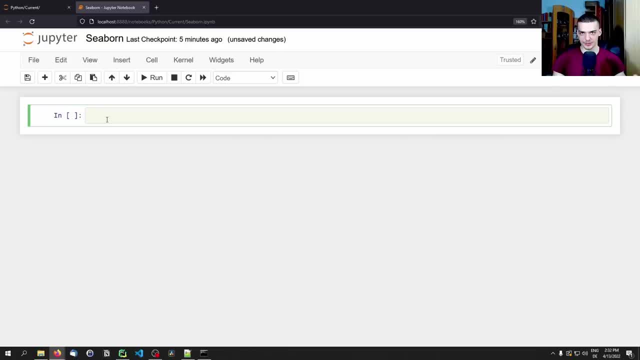 the same Python code that we write today in the Jupyter notebook, also in another development environment, but it's more convenient to use an IPython notebook. So, having said that, the first thing we want to do is we want to install Seaborn, And for that we open up a command line and we 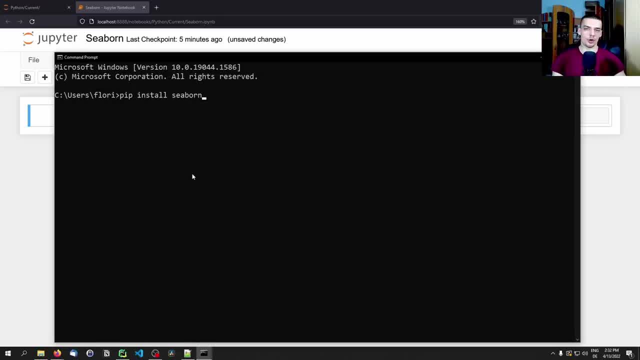 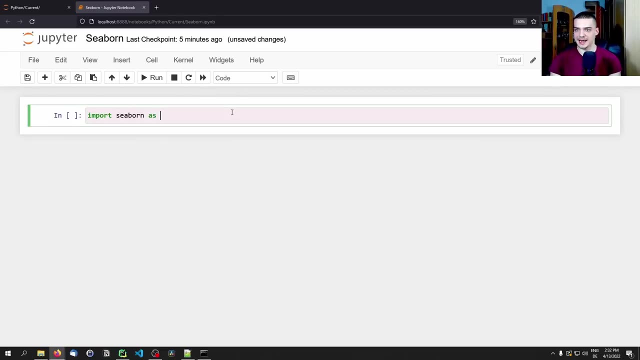 type pip: install Seaborn. If you are using an Anaconda environment, assume you already know how to install packages, usually with conda. install Seaborn, Even though you can also use pip there if you want to. Once we have that, we can start by importing Seaborn s SNS. 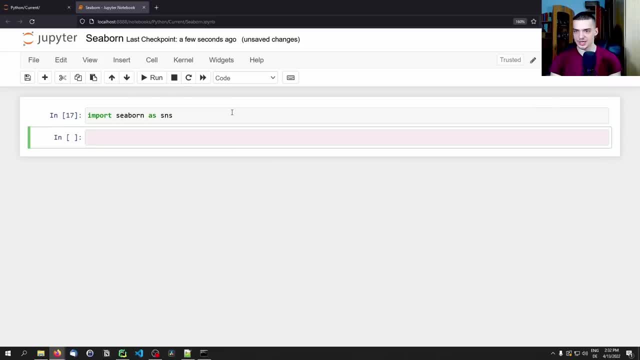 which is the usual alias, And then we can just get started with some data sets, Because for the visualization we need data sets And you can use whatever data set you want. I'm just going to talk about general visualization functions here. You can use a data set from Kaggle, you can use a. 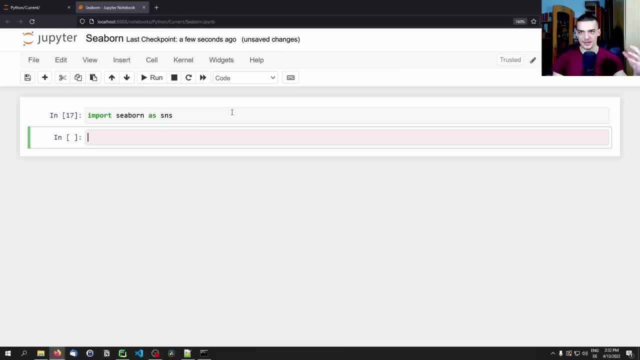 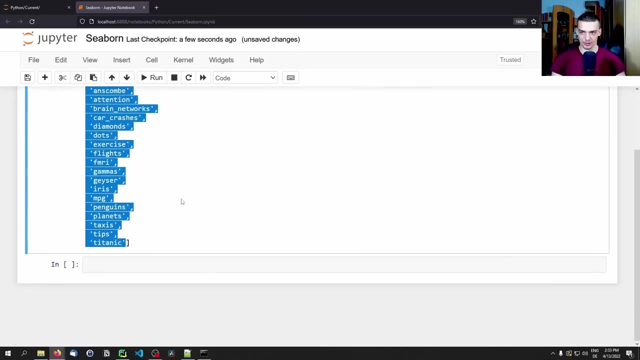 CSV file that you have on your computer. you can use stock data from the pandas data reader if you want to, or you can also just go ahead and say SNS, get underscore data set, underscore names, And you can pick one of those data sets that are provided by Seaborn automatically or built in here. 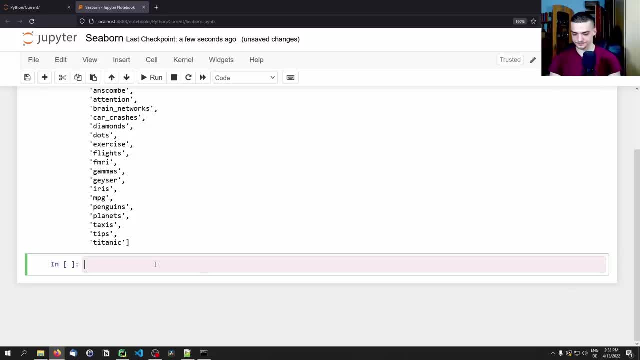 And we're going to just load a couple of them here. we're going to say: tips equals SNS- load underscore data set Tips. then we're going to say iris equals: load iris. Then Titanic- load Titanic. And then planets- load planets. just so we have some data sets here, And the first one that we're going to 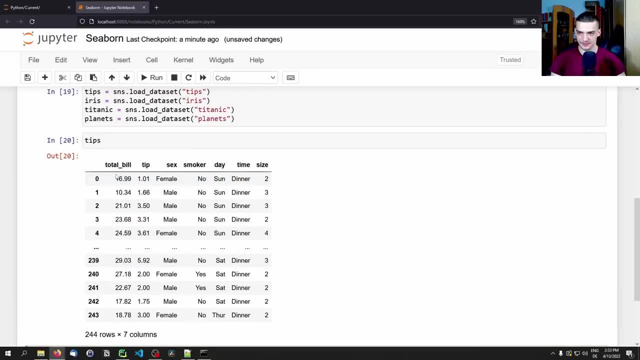 look at is going to be tips, So we can just type tips And we're going to see here, as a pandas data frame, what this looks like. we have the total bill, we have the tip, we have the sex, we have the smoker. 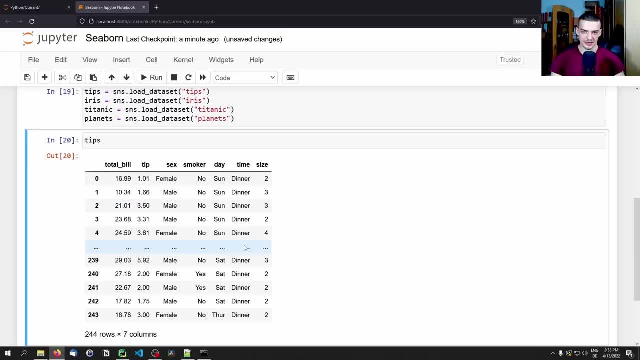 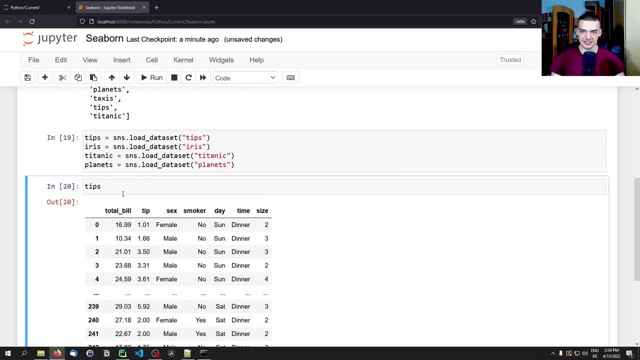 yes, no, we have the day of the week, we have the time when, when this meal was consumed, and then we have the size of the meal at the restaurant. So this can be used for tip prediction. whatever, we're not going to do any machine learning Today. we're just going to visualize the data And the 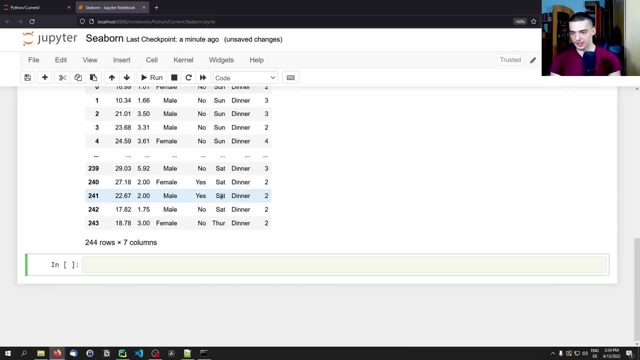 first thing that we can do here is we can plot a simple scatterplot by saying SNS scatterplot, So basically just the individual data, And we're going to say that the X value that we want to plot here is the tip. So how much was tipped? 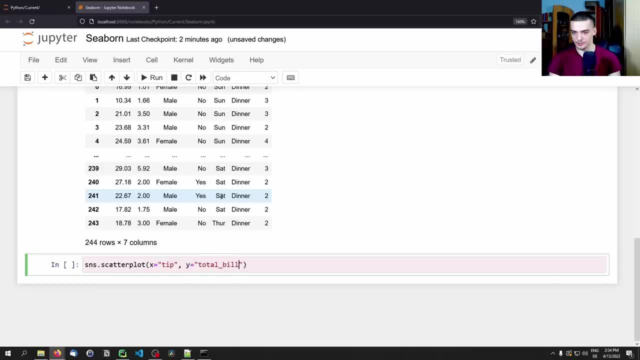 whereas the y is the value of the total bill. The data set is the tips data set that we loaded here, And then we're going to also. first of all, let's, let's just do it like that, So we can see a very 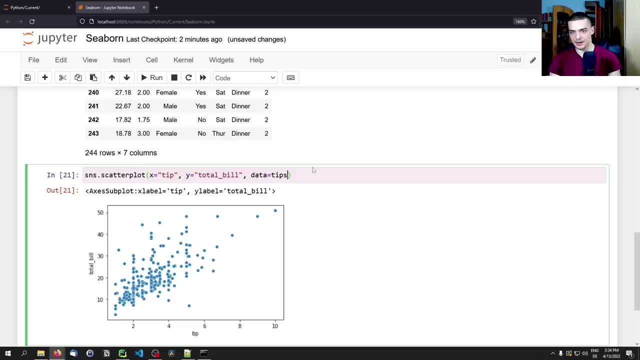 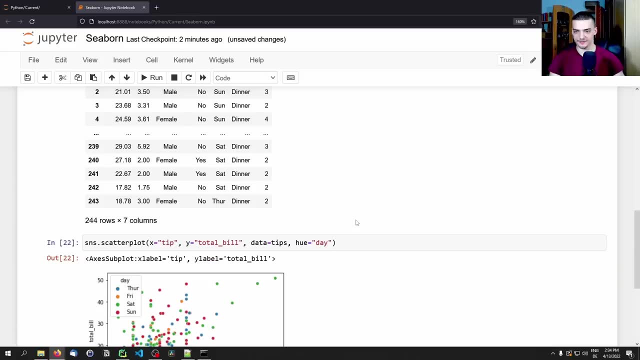 simple graph like this one here. Nothing fancy about it, But now we can do something like hue, And this is going to be the day this year, And now we have categories represented in colors, So now you can see. okay, if it's. 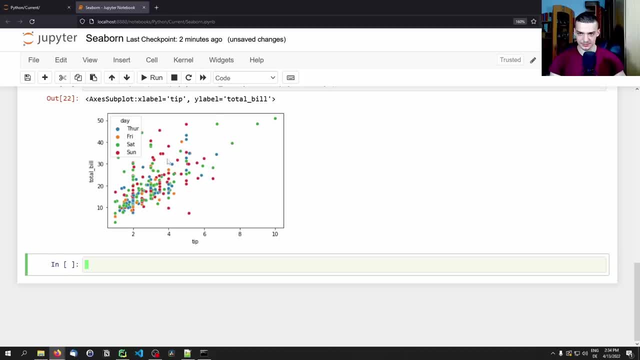 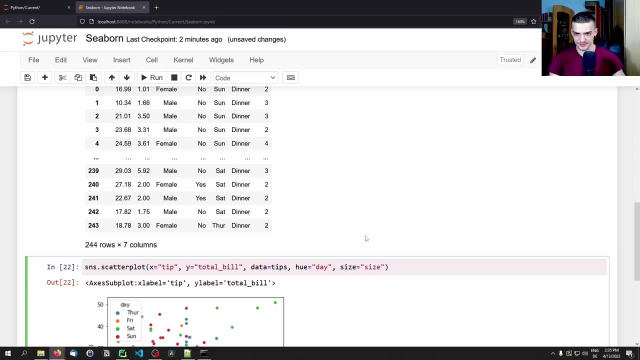 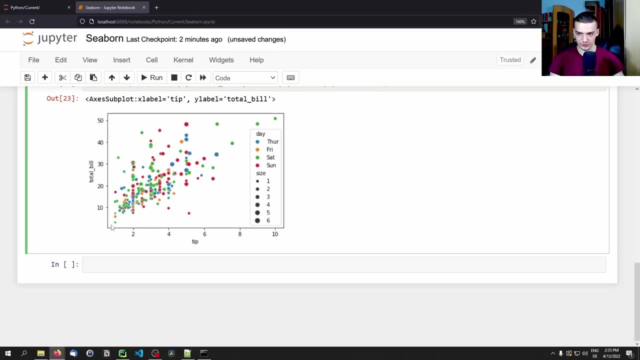 Saturday it's green, if it's Thursday it's blue, and so on, And we can add some more information. we can say, for example, the size of the individual data points is the size of the data set. So, depending on the size of the meal, we're going to change the size of the individual data. 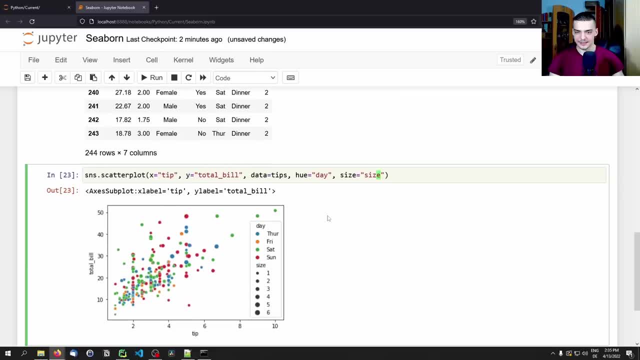 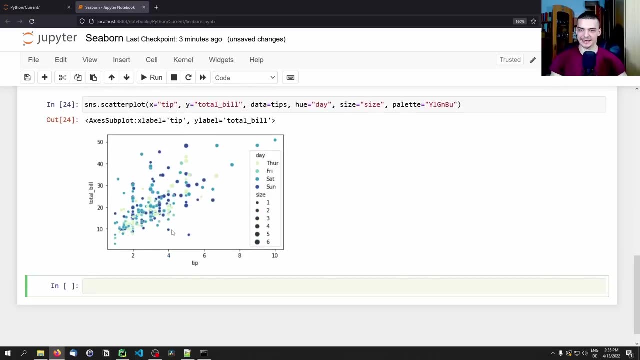 points. So this is a very small meal, this is a larger meal, And then we can also change the color palette- I hope this is how it's pronounced- And this is going to be yellow, green, blue, like that. And now we can see. this is already quite an informative visualization And we didn't have 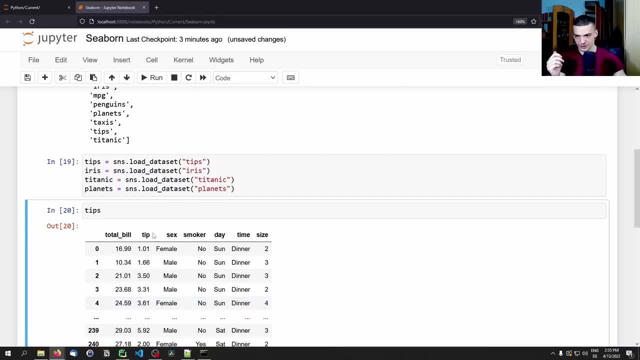 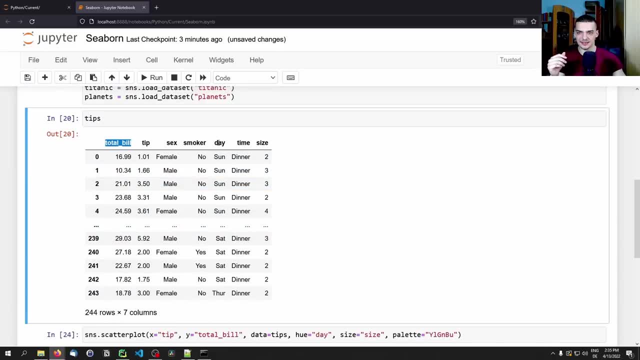 to really do anything. we just said: okay, x value is a tip, which is numeric, then the y value is the total bill, which is also numeric. So quite simple To plot on a coordinate system. And then we just passed the day, which is a categorical value here. 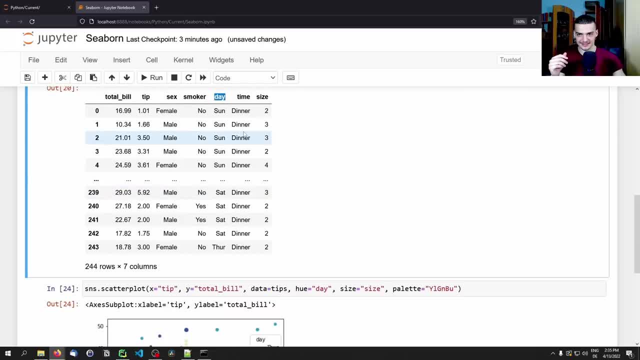 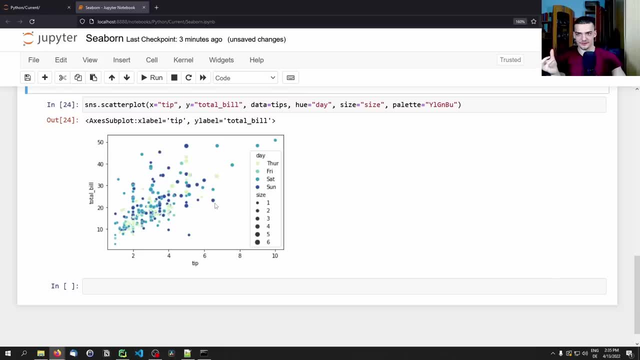 and it's now determining the color. And then we pass the size, which is a numerical value, to determine the size. So we didn't have to really think about how to do something. we didn't really have to spend a lot of time looking up certain conventions or anything, or certain functions that 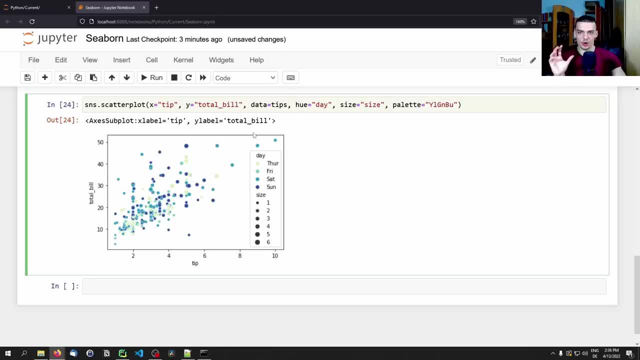 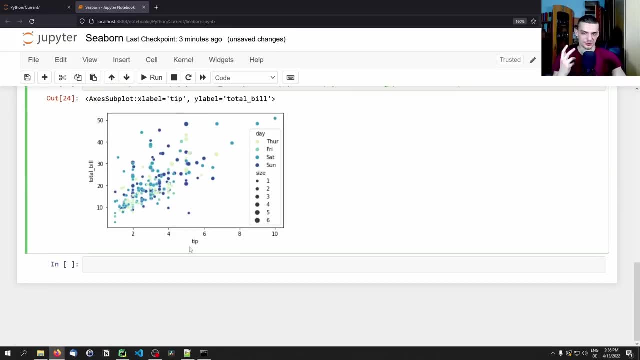 we have to use. we just pass the individual fields and Seabourn automatically generates a very informative scatterplot. Now we have different types of plots, So this is probably the most simple one. for me, a scatterplot is always the most simple plot. 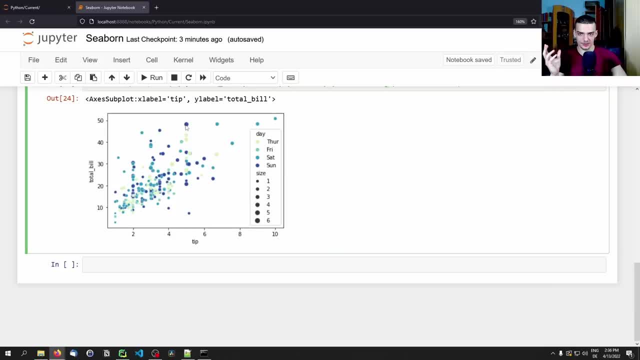 possible because we basically just take two coordinates and we point, we plot a single point, a single data point, and then we do that for all the rows. But we also have some more statistical type of plots, like histograms or distribution plots, And for that we can for example say: 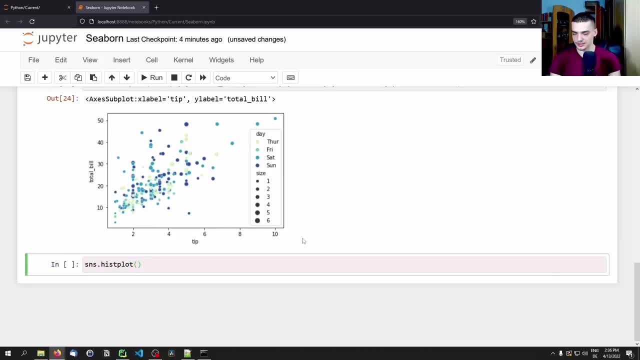 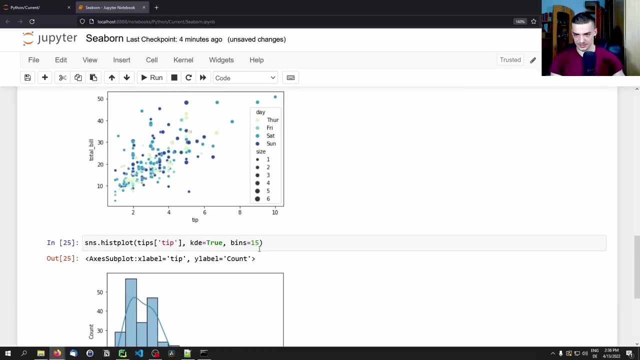 sns dot hist plot, so histogram plot, and we pass your tips, tip. So we're interested in the tip, all the tips, and we're going to say, Katie, equals true, to get the line as well And we can specify the bins of the histogram. So in this case, here 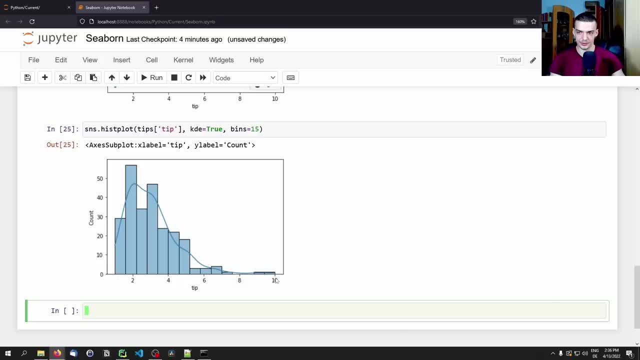 this is the distribution of the tips. very few people give a tip around that value, So now I think tip is in dollars, right? So we don't have a lot of people tipping $10.. We have very many people tipping around $2, or three or something like that, between $2 and $3. So we have a lot of. 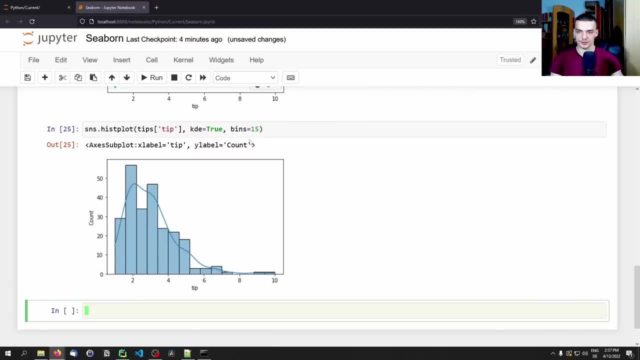 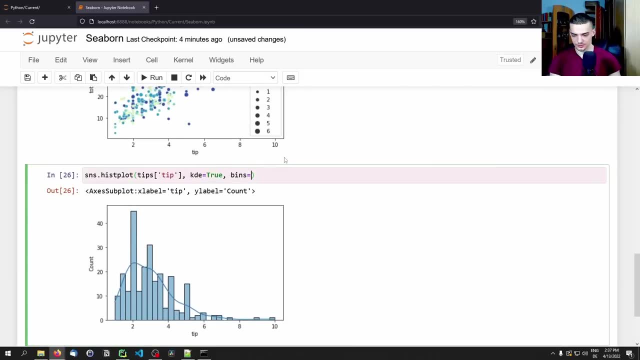 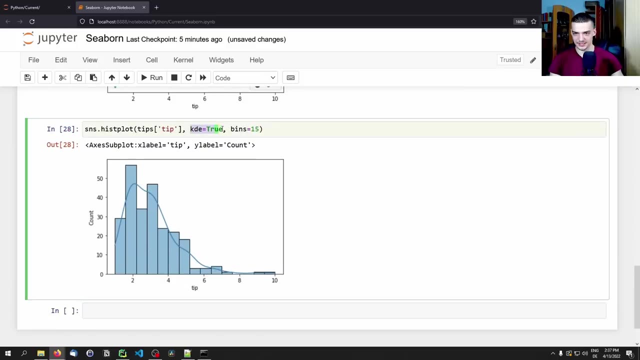 people tipping around $2 and $4, basically, And we can see here the distribution function. we can also see more if I say bins equals 30,. we can see more bins If I say bins equals five. we're going to get less information here. I think 15 is quite a good value, And if I say 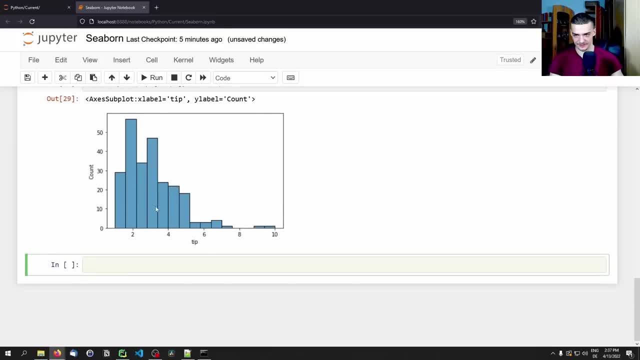 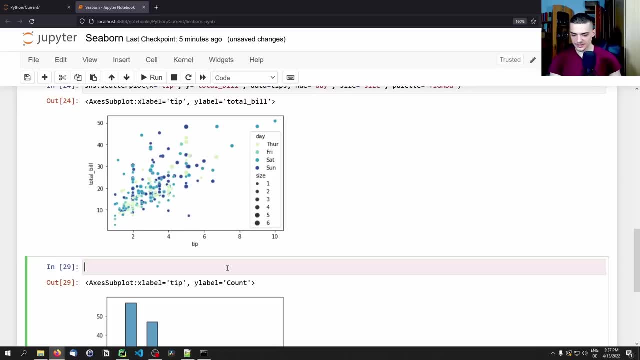 Katie equals true, is no longer the case. we don't have this line here, this function, So this is a very simple one. we can also plot it in a different way, though, So I can also say SNS dist plot for distribution plot, And I can pass the same value. So, tips, tip. 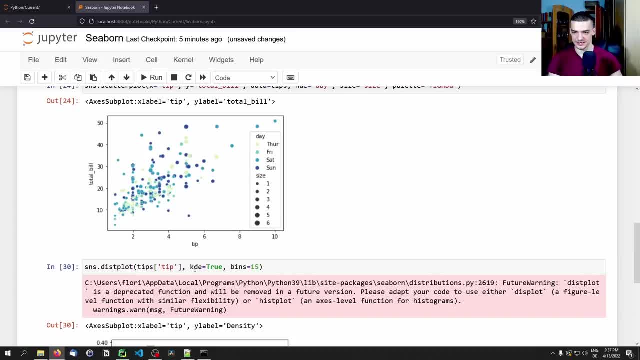 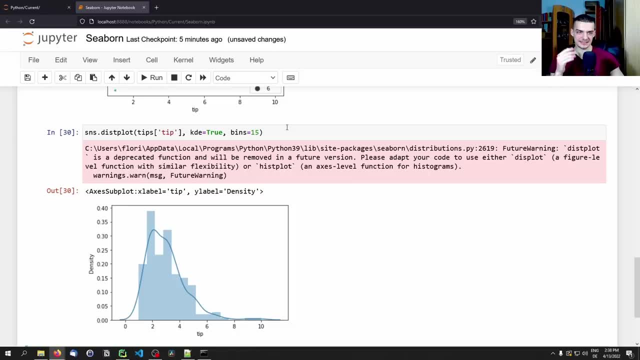 Katie equals true and bins equals 15.. And this is almost the same function, even though what does it say here? future? Oh yeah, it's a deprecated function. That's why we have the same function. So don't use the dist plot function, use the hist plot. But right now I recognize actually the T. 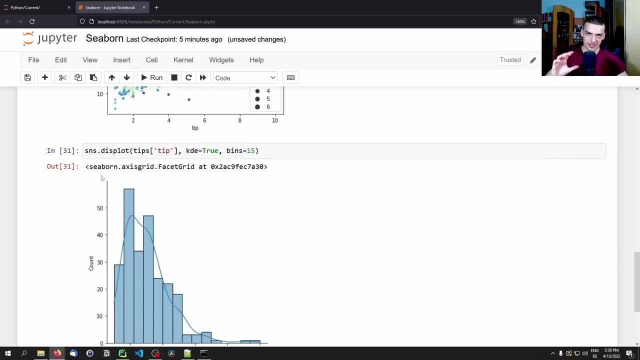 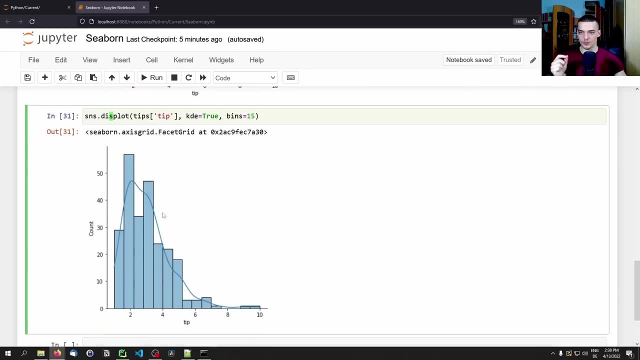 is something I didn't want to have here, because we have the dist plot, which is deprecated, we have the hist plot, which is not deprecated, And we also have the dis plot without a T, which is essentially very similar to the hist plot. So I can actually copy this here and change this. 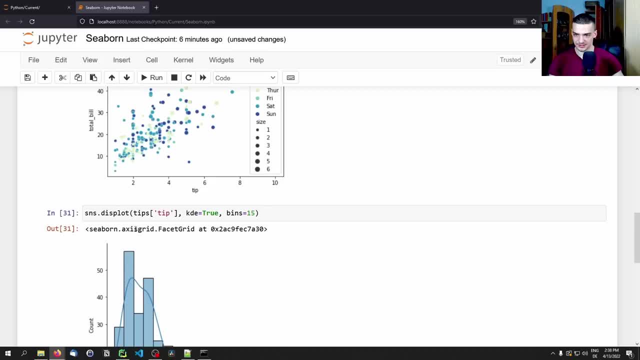 back to an H and add a T, And you're going to see that they're quite similar. This one is a little bit larger when it comes to the vertical line, But essentially they're the same plot from the information. Now then we also have the dist plot, which is a little bit larger, but essentially they're the same plot from the information. 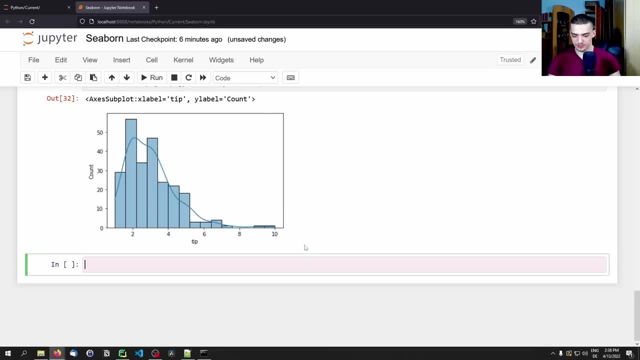 barplots. barplots are very, very simple plots as well. we just say SNS barplot And then we can say: okay, on the x axis, I want to have the sex, so male or female. on the y axis, I want to have the tip. 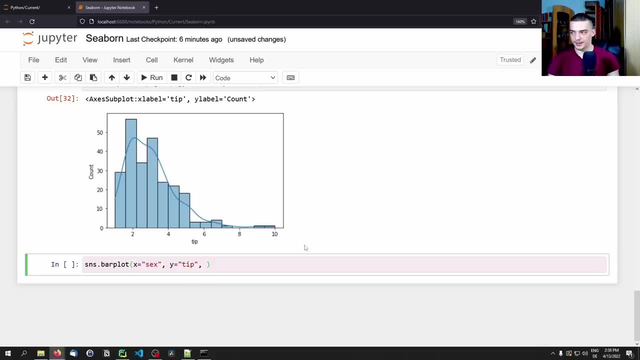 so we can see if there's a difference between the genders And then we can say the data is tips And the palette is going to be yellow, green, blue, like that. So this gives us some information. we can see that on average. we can see that we have about eight out of 10, maybe something. 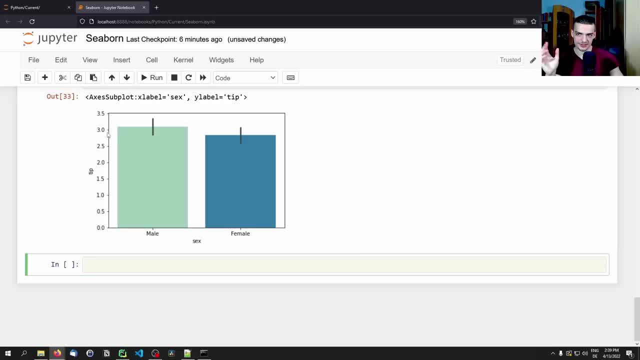 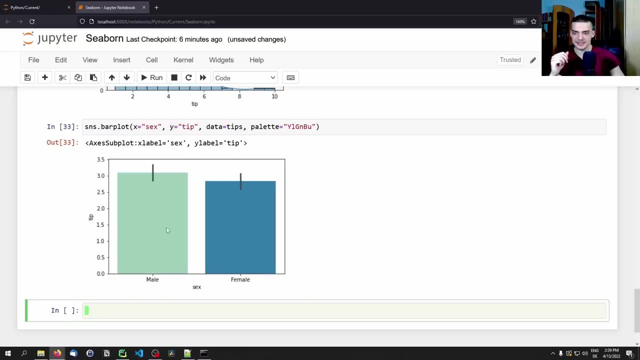 we have a slightly higher bar on males, So males seem to give more tips usually, But this could also be because males maybe eat larger meals. We don't know yet. So this is not something that we can see in that visualization. That's a very, very simple bar chart. 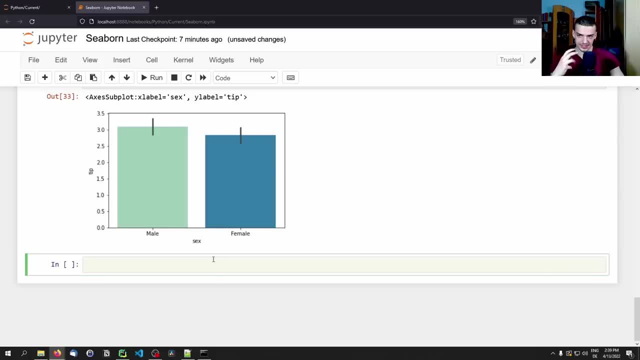 A more complicated statistical chart would be a box plot, which can easily be plotted with Seaborn as well by just saying snsboxplot. And here we're going to say, okay, now we want to see what the distribution of tipping is on particular days. 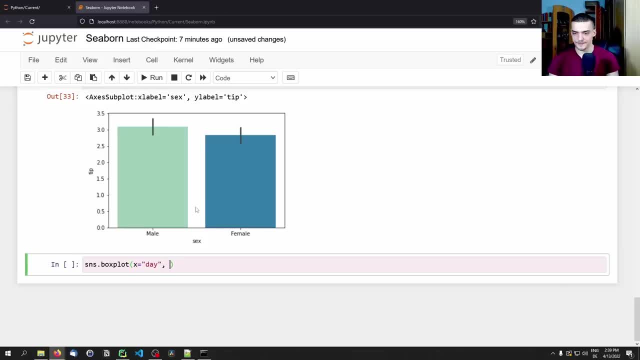 So on Saturday, Sunday, Friday and so on, Compared to the total bill data is tips or actually we want to in this case, let's change this to tips. In this case, we'll look at the tips. Otherwise, we'll look at the meal size or actually the total bill amount. 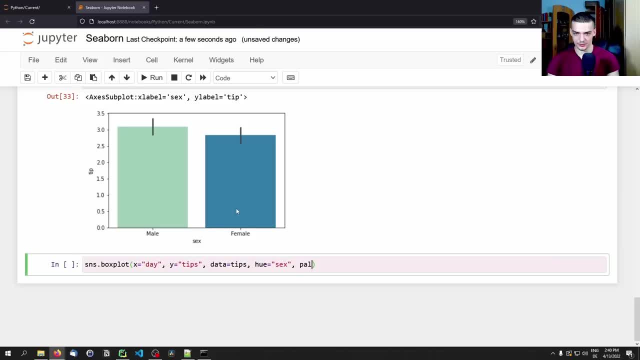 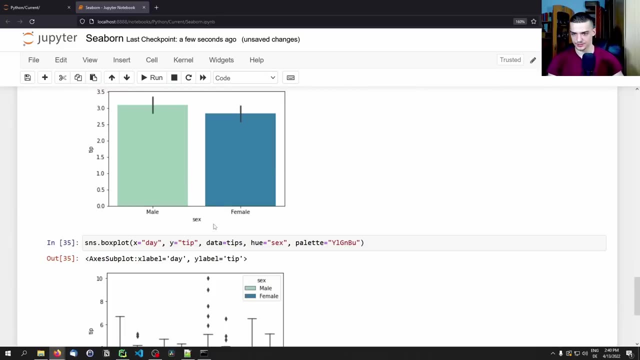 And the color is going to be the gender, And then we're going to choose the same color scheme here: Yellow, blue, green, Actually green blue, Sorry. And we have a problem here. Tip, I think Tip without an S right. 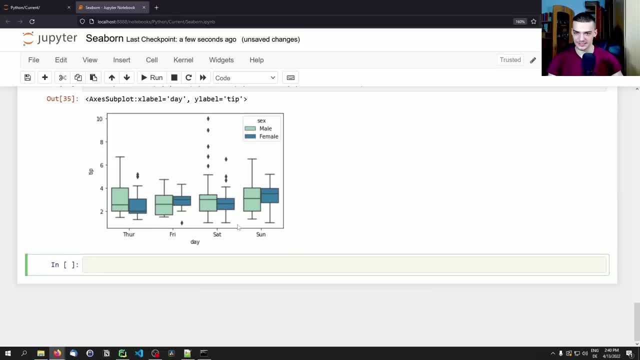 There you go. So you can see here that on the different days we have different distributions. We can also look at the total bill, which is probably not too different, But we can see, for example, that the center line- here- for those of you who don't know how to read a boxplot- 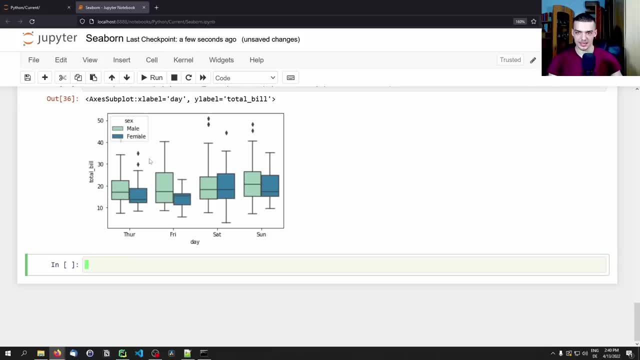 this is the median, So the center value, those are the quartiles, And so, basically, the quartiles are the four sections of the boxplot. This is the maximum, This is the minimum, And then we have some outliers that are not considered. 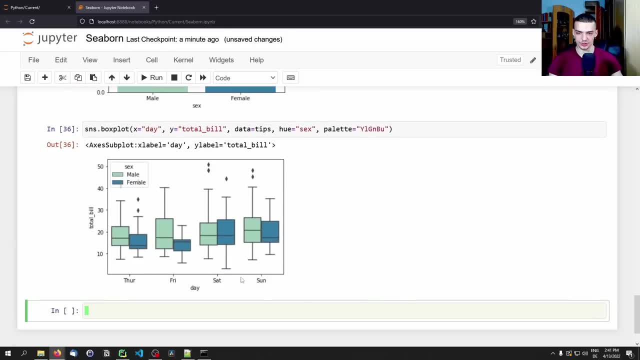 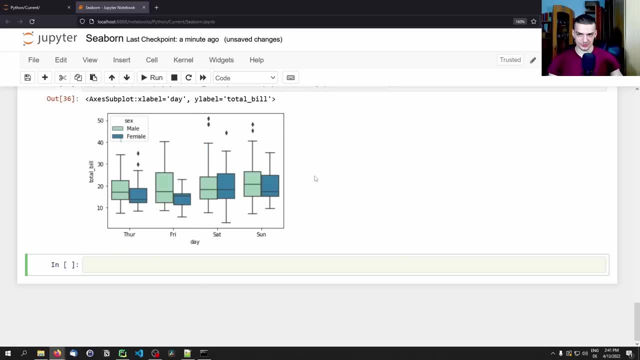 But here you can see how easily we can plot the distribution. Also, blue meaning female and green meaning male. That is quite simple in Matplotlib 2.0. So we can see how easily we can get this plot with that information. It would be more complicated. 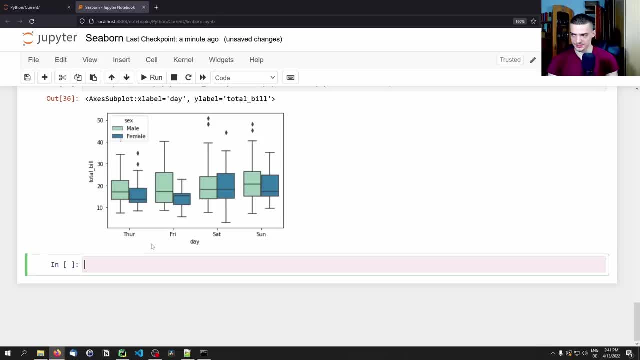 So Seaborn makes this way easier for us. We can also plot something similar, even though it's not exactly the same as a boxplot. We can plot a strip plot, So it doesn't have information about the quartiles and the medians. 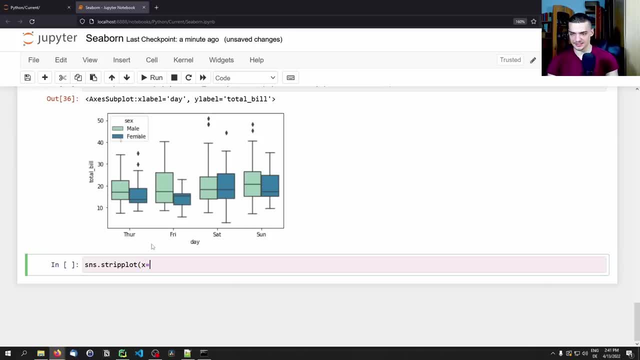 But we can see the distribution of the data points easier. So we can say x equals day, y equals tip, for example, And then data equals tips again, And we're going to say dodge equals true. Dodge equals true is important because let me show you what happens if we don't do that. 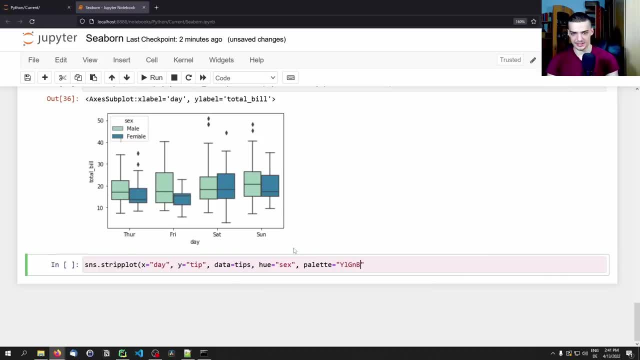 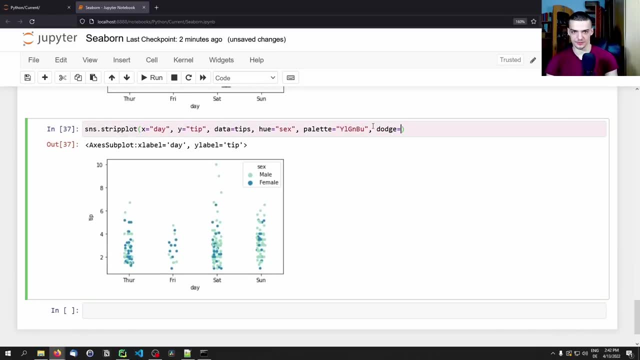 And then we're going to set the same color scheme, So yellow, green, blue. So this is what happens if you don't dodge. And if we now set dodge equal to true, we can see that the genders are separated. And now you can see the distribution of tipping. 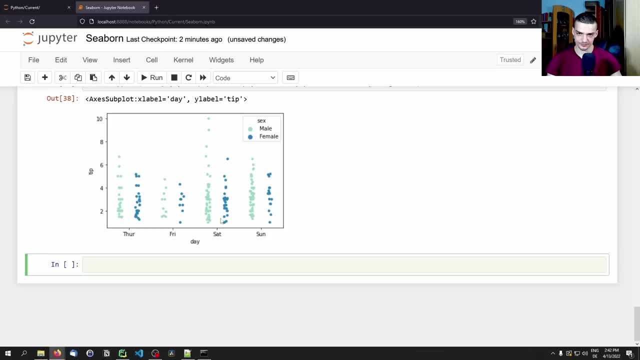 You can see that males usually are higher. you could say So on Saturdays. we have a lot of high tips that are coming from males here as well. Actually, for each weekday this is the case, even though we have also some males that don't really tip a lot. 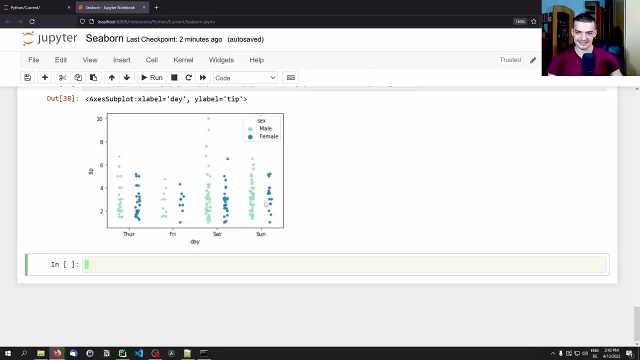 which is, yeah, at least on Friday and Sunday. it seems like this is not the case for females. We have fewer females down here, even though they always occupy- I'm not sure about Saturday, but other than Saturday they always occupy- the minimum position. 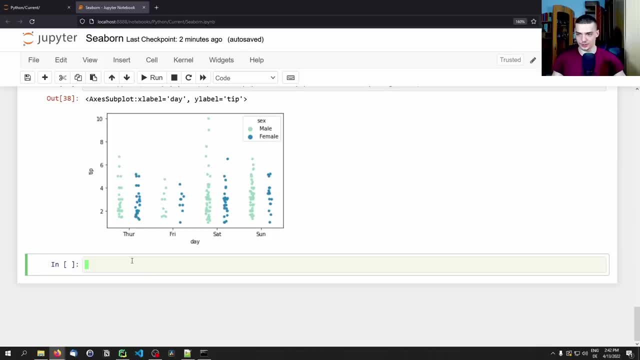 So one could further examine that if we were doing some data science work here. Now let's get to some more complicated plots, because those are still quite simple. Let's do some joint plots, which are essentially a scatter plot and a distribution plot at the same time. 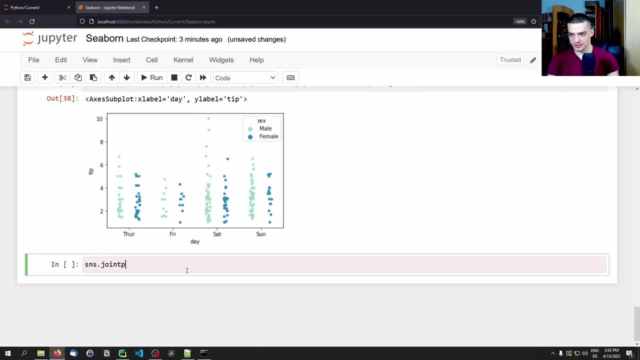 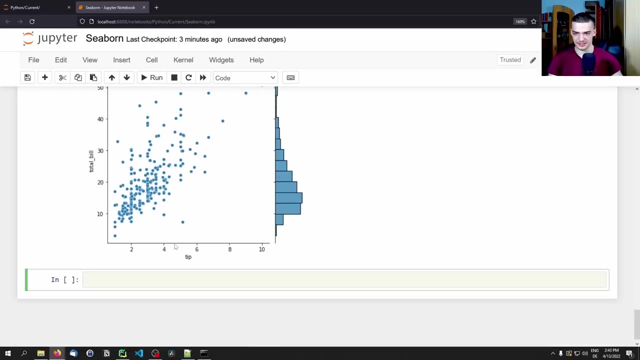 So what we do here is we say S&S joint plot And the X value is, for example, the tip, The Y value is the total bill And the data is tips, And then we can just plot this joint plot here And what you see is that we have a scatter plot. 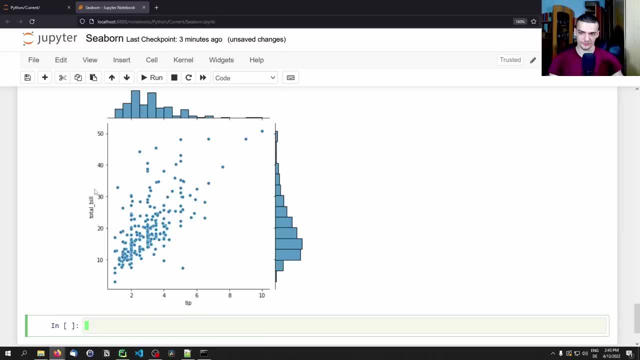 And also we have 40 individual features. so for tip and for total bill here, the distribution function. This is quite interesting of a plot to look at because it's a combined plot And again the main focus on Seabourn is always. it makes it easy for you. 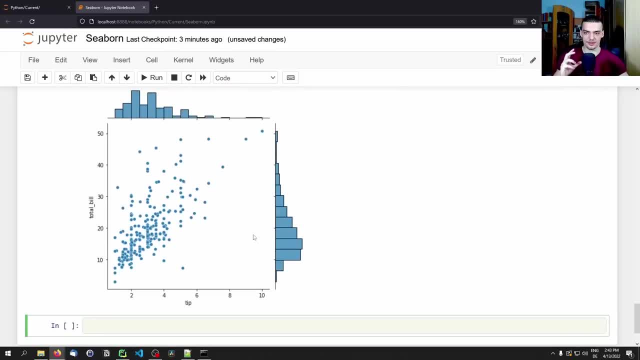 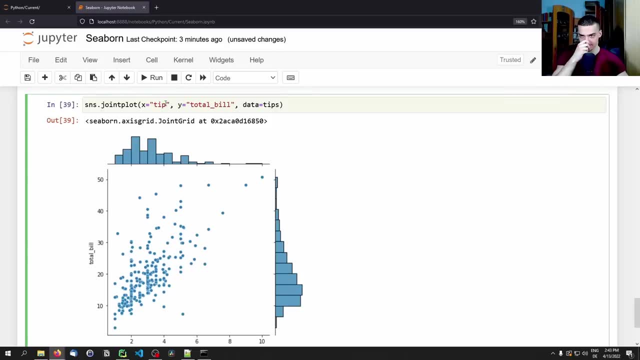 Everything you do here with Seabourn can be done in Matplotlib as well. The main emphasis here is how easy it is to do that. You just take a data set, You just set some values here And then you get very good looking and very informative plots. 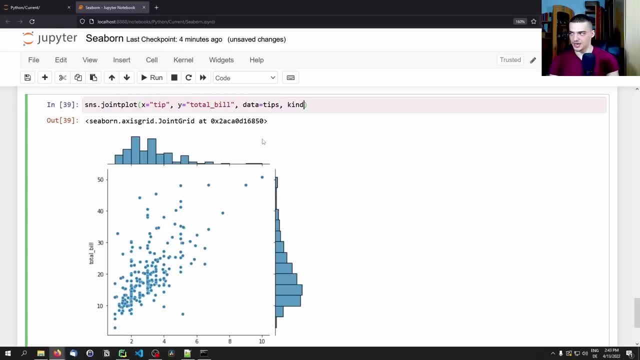 Now we can add some more stuff to that. We can also say: kind equals rec for regression, And then we see here a regression line and also the distribution function here as well. So this is also quite simple. Now, I haven't played around with that. 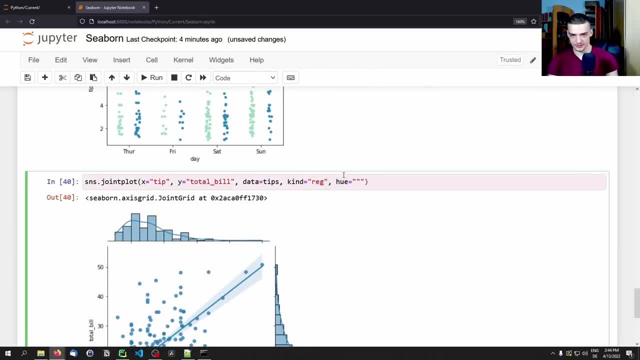 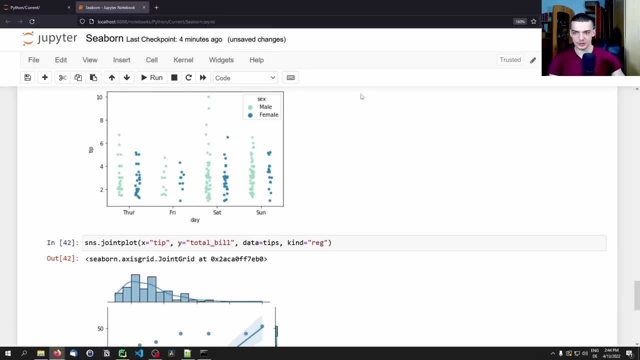 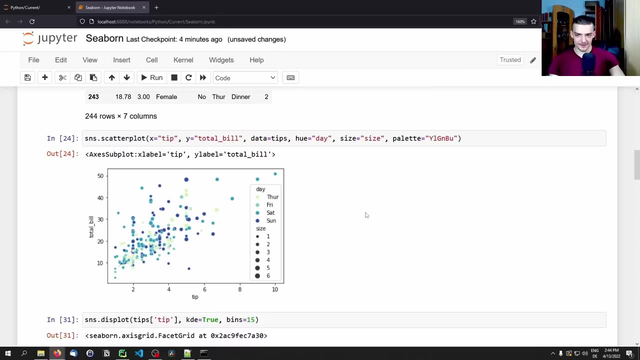 but maybe we can also determine the color here. I'm not sure. No, it doesn't work in this case. Maybe there's a different keyword for that. But usually you just look up the documentation. You see a bunch of different options and usually it's enough to just specify a column of some of the features here. 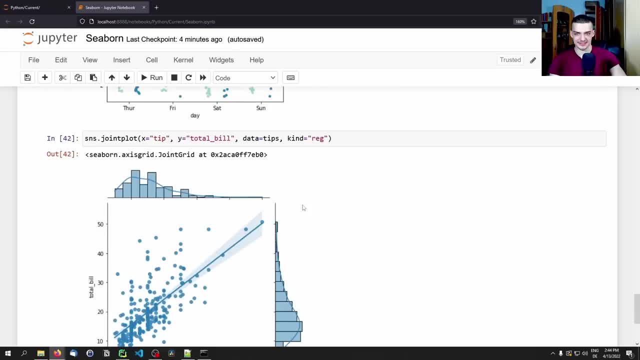 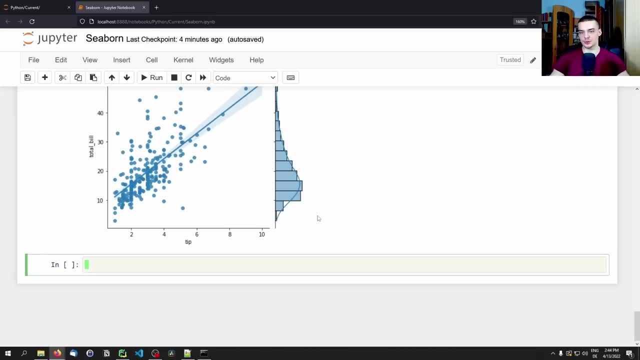 So basically just taking something like size or time, and this is going to already be translated automatically without you having to turn it into numerical values first or something into a color, into a size, into something like that- Now we can also change the color. 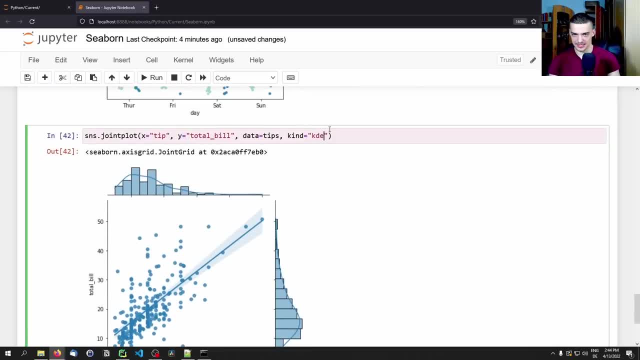 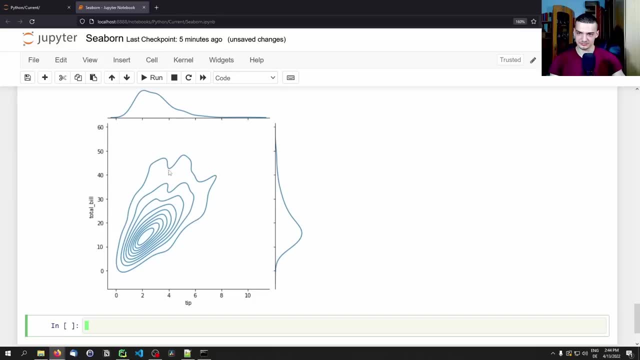 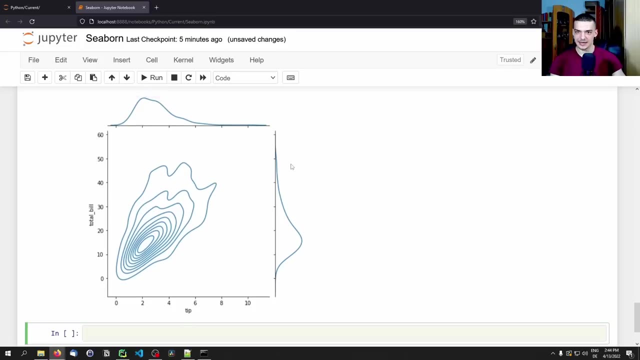 So we can say kind here from regression to KDE, And this then turns it into something like that: This is more like a three-dimensional plot here, where you can see: okay, the main concentration is here, And then the further out you go, the less instances you have here. 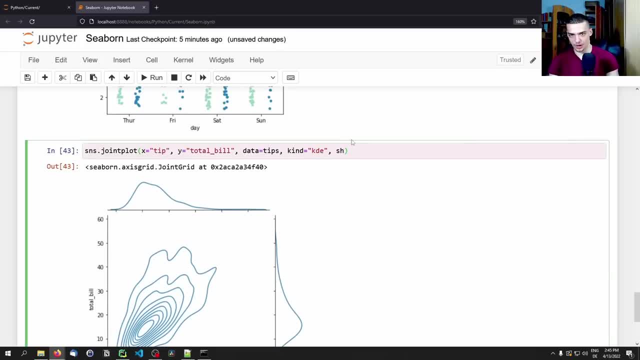 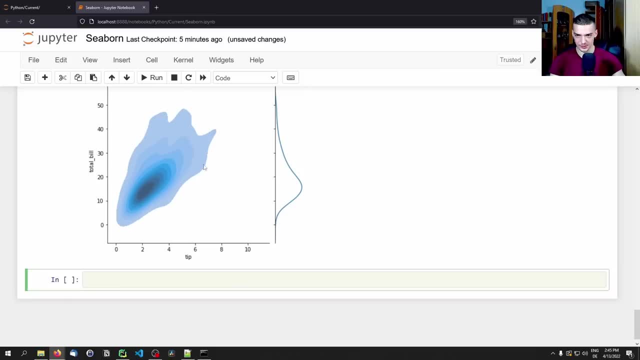 Now, if you want to see this better or more obvious, you can also set the shade to true. Then you can see where the concentration of values is. So here we have a lot of values, Here we have less values And here we have no values. 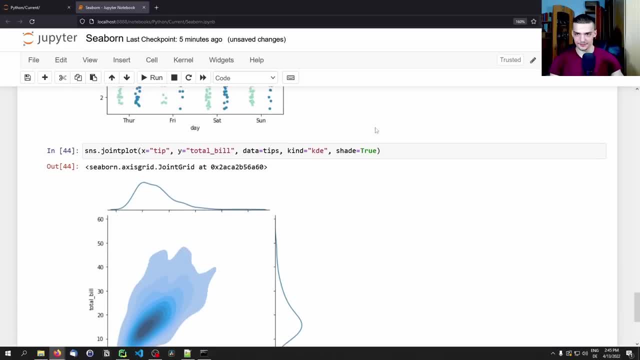 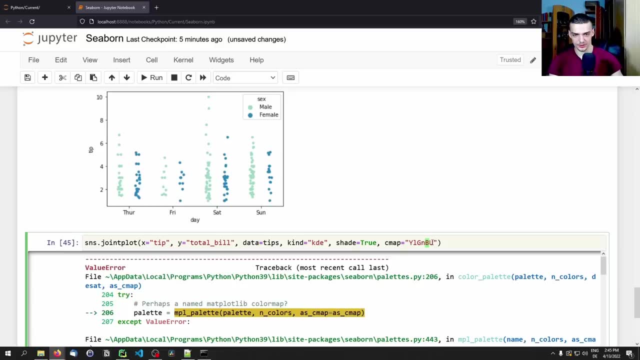 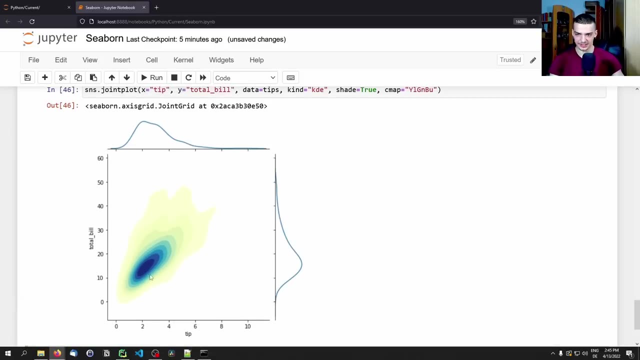 Basically, And that again can be influenced by setting a color map. So color map equals yellow, green, blue, again with a lowercase u, And you can see here that we have a pretty good looking plot that shows us that most values are here. 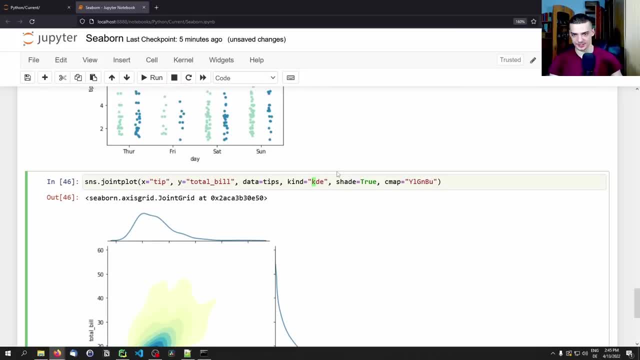 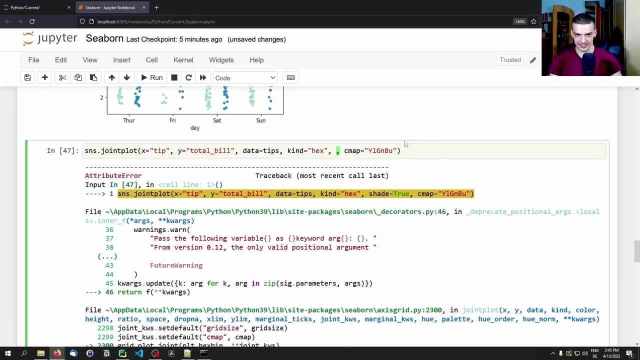 Now we can also change that slightly by changing the kind here to hex. Now we have hexagons. Actually, what's the problem here? We don't have shade in hexagons and hex plots, So this is basically the same thing. 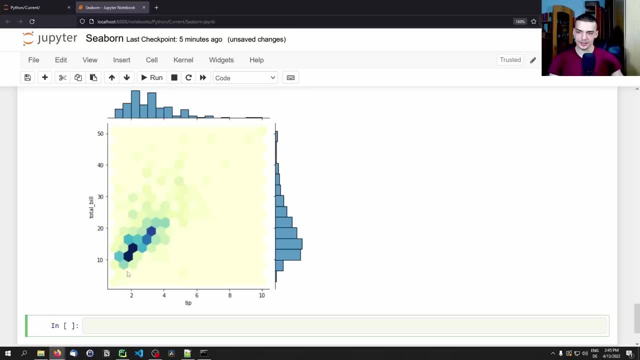 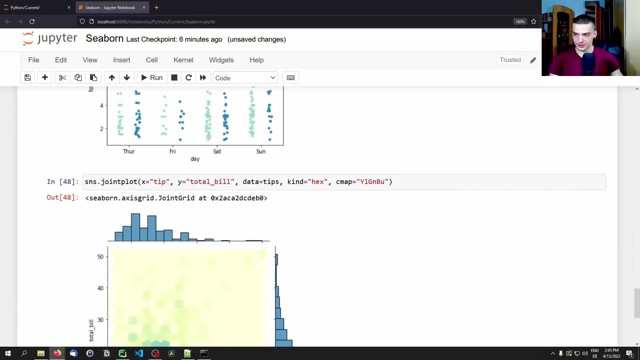 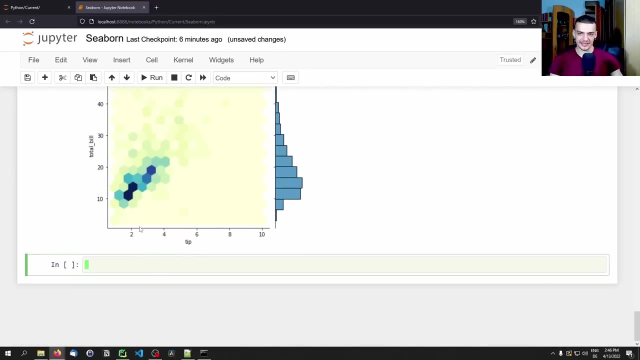 We have most values here, here, here, here, here, But now we have this as hexagons, So this is also quite interesting. All sorts of different plots here. Now, one of the more complicated plots or one of the more bigger plots is a pair plot. 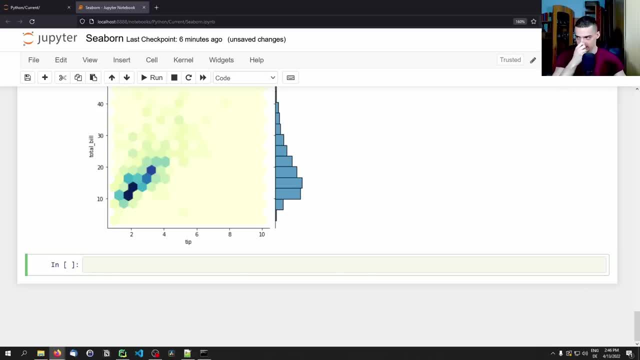 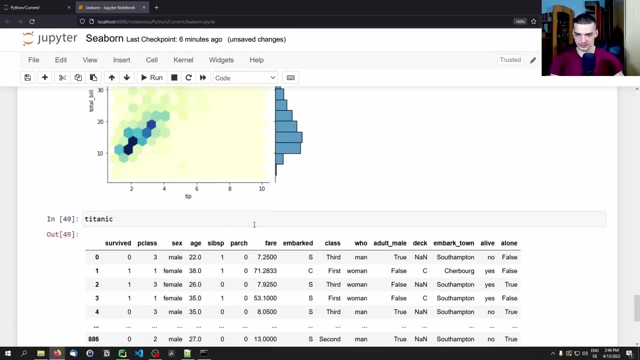 Basically combining the individual features in a pair plot. How can this be done? We can just say snspairplot And then we can pass a data set. for this one, It probably makes sense to not use the tips. Let's see what the titanic data set looks like. 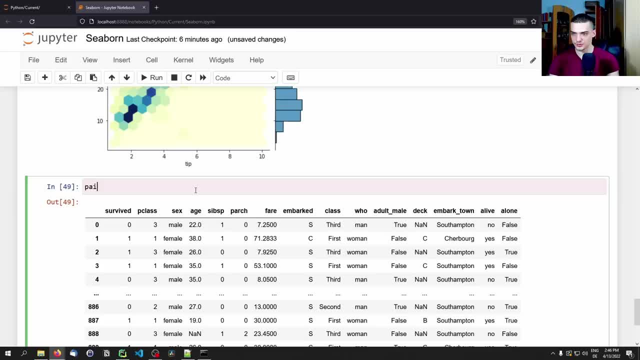 Yeah, This looks like something that can be quite interesting. So pair snspairplot And then titanic, And we're going to just select the numeric values, because we cannot use categorical values here. So select underscore d types number to just get the numerical values. 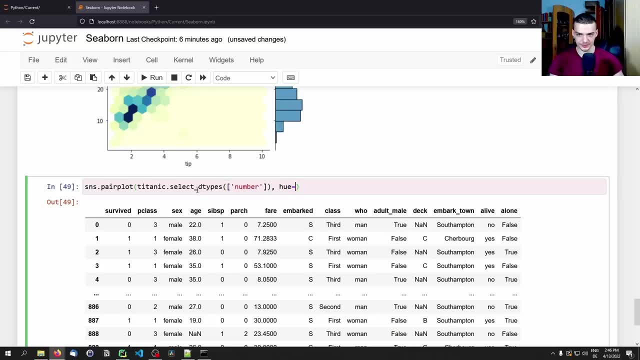 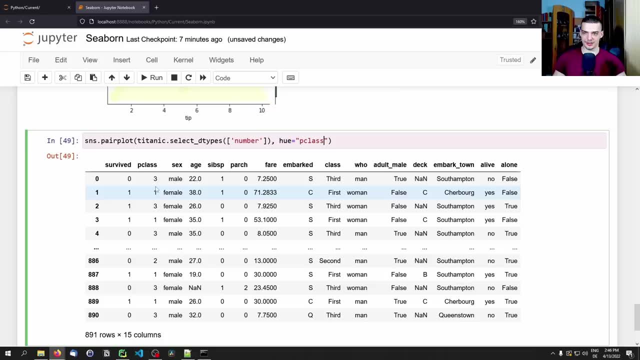 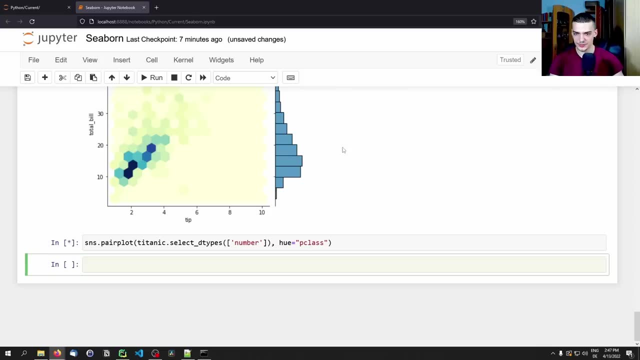 And then the color is going to be determined by p class. For those of you who have watched my titanic video, the data set analysis here, they know that the class of the person is very highly correlated with the survival. So if we do that, we can see here a pair plot. 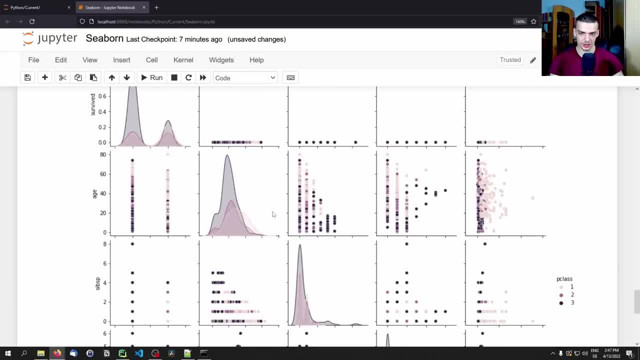 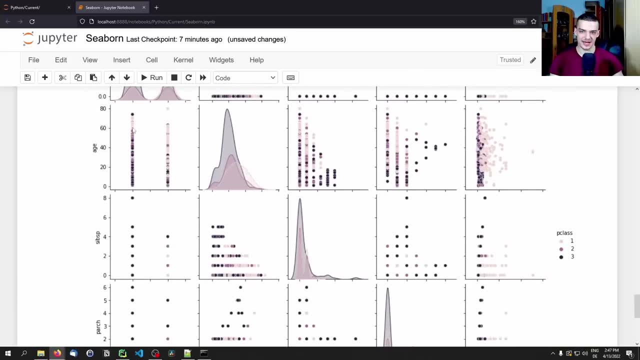 Which is quite a large plot. You can see here the different features plotted against each other. So we can see: survived and survived Whenever we have the same value, so the value plotted against itself. it would be just a straight line, So a correlation of one. 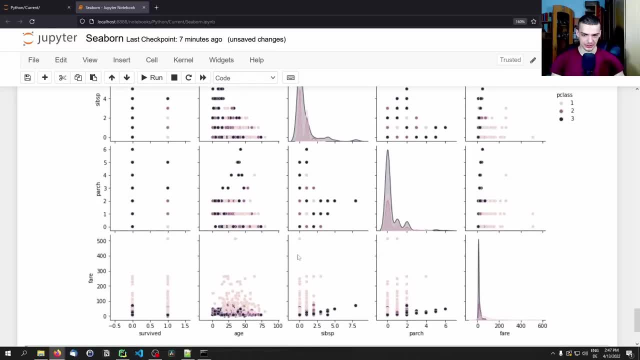 Because of that, we get a distribution function here, distribution plot, And for the other values, we have the values plotted against each other, Which is quite cool. Now, then, we get to one of my favorite plots, which is one that I use in a lot of my videos. 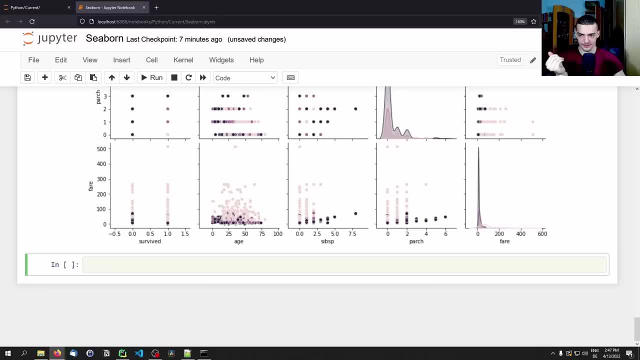 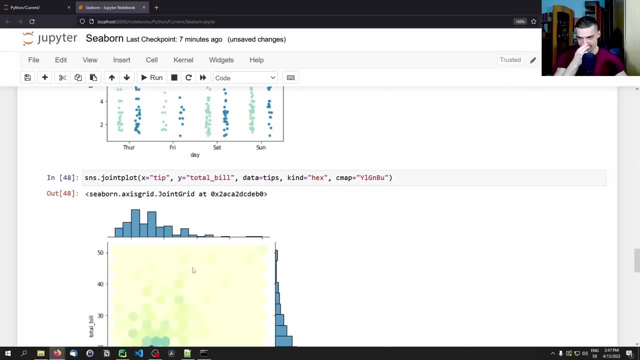 And whenever I explore a data set for prediction of something, I always use that because that is really something that's very important Whenever you have a data set- like the titanic data set, for example, where you want to know how can I best predict a survival. 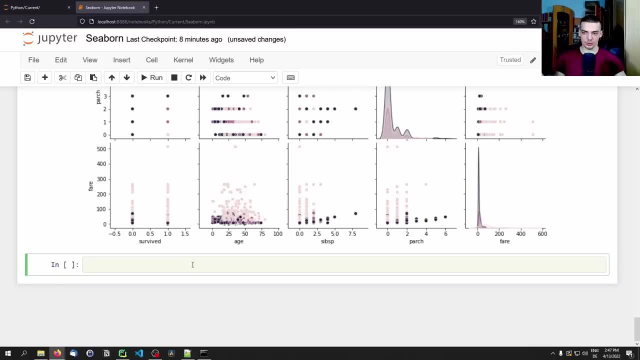 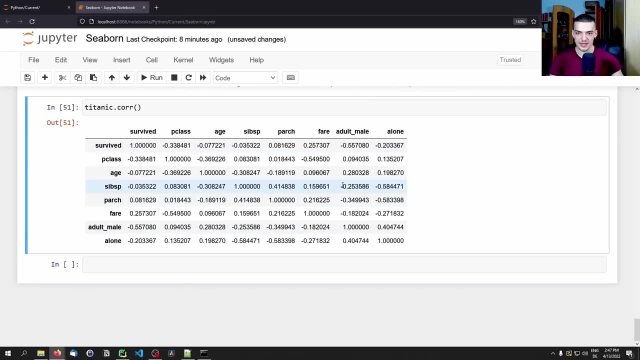 you want to look at correlations, And when you look at correlations, when you have a data set like titanic, for example, you can call the core function to get the correlations between the individual values, And this is fine, because here you already have all the information you need. 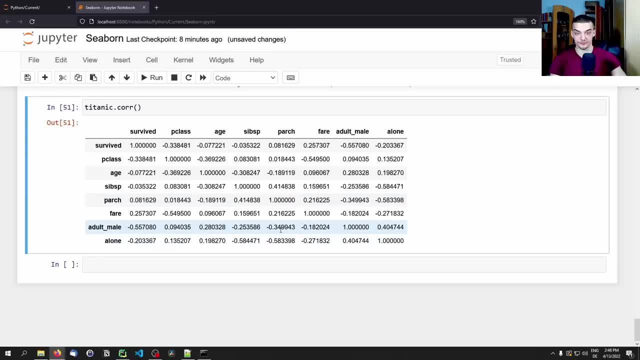 But it's very hard to find the values, especially if you have more features than that. It is not a good overview because you just have numbers and you really have to look for numbers here. It makes more sense to put that into a heat map. 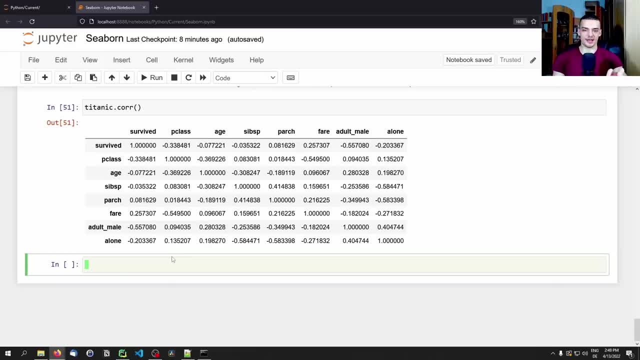 A heat map is basically showing you where you have high values by showing you colors. So let me show you what that looks like. We can just say snsheatmap and we're going to pass here titaniccore for the correlation We're going to set. annot equals true. 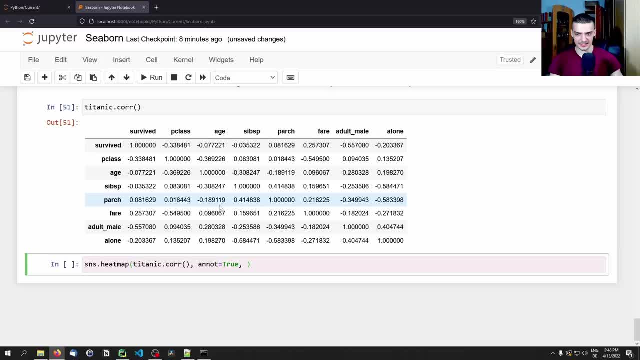 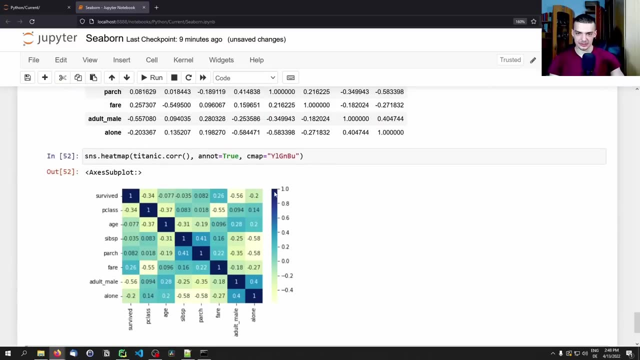 So the annotations. This basically just means we're going to also see the numbers, And then we're going to say the cmap is going to be yellow, green, blue again, And then you have this very beautiful heat map. Whatever is closer to dark blue is highly correlated with each other. 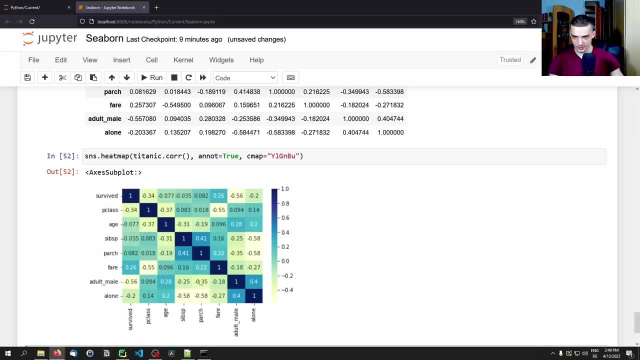 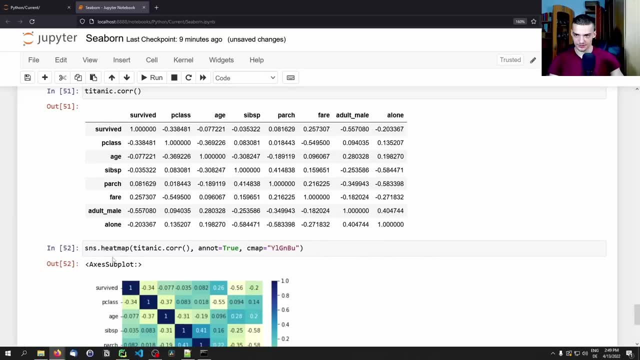 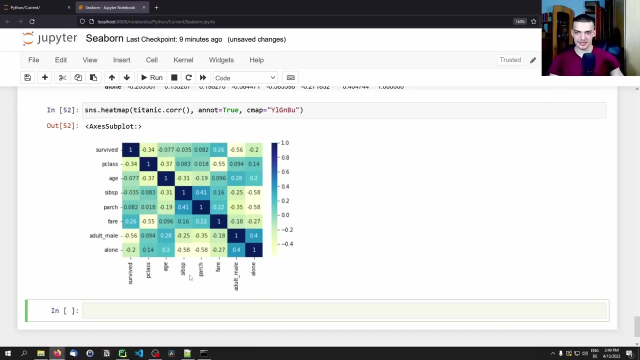 So if we have, for example, something with this very high correlation, something like 0.41,, this means that the siblings and what was PR, I think parents, children- is highly correlated. So if we have someone with siblings, they probably also have parents or children, or something like that, on board. 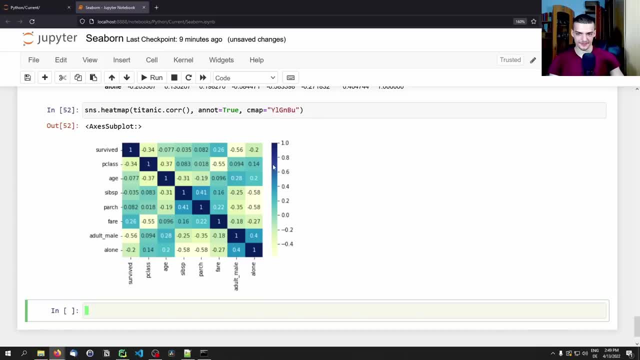 And negative correlations are also important. So when something is highly negatively correlated, it's also interesting, because that does not mean it's irrelevant. Irrelevance is close to zero. That basically means there is no correlation. Negative correlation also gives us, gives us information. 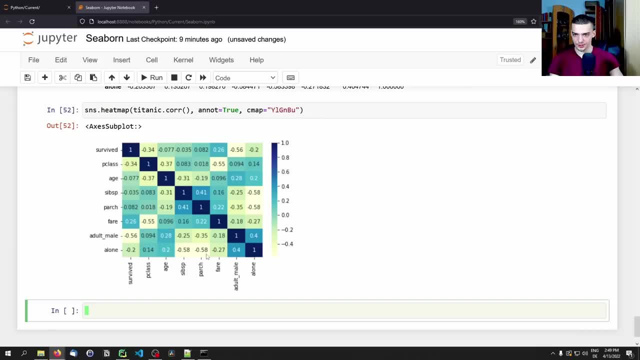 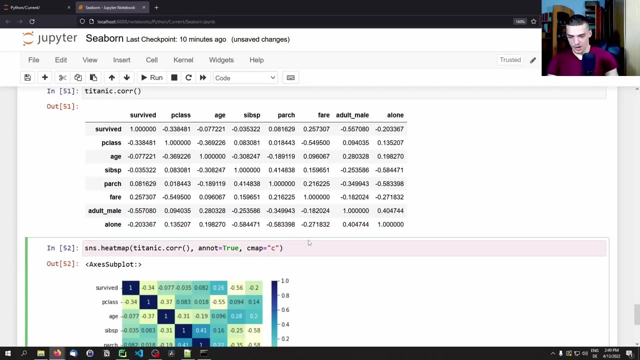 So, for example, we have something like 058 here, and this is negatively correlated to alone. So when you have parents or children, you're probably not alone, obviously, Or something like that. So we can also use other color maps, like cool, warm here. 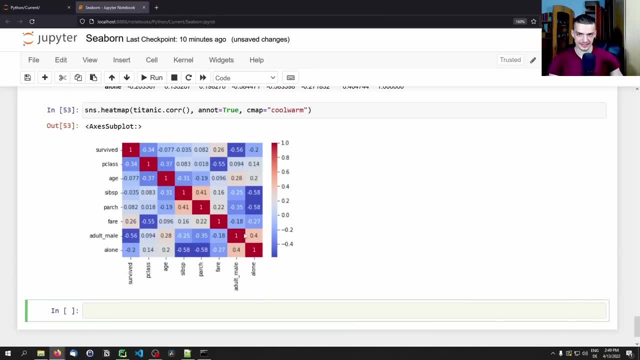 which might make more sense. The hotter something is, the more correlated it is, the colder it is. So the more blue it is, the less, the more negatively it is correlated, And the more white it is, or gray, the more it is close to having not any correlation at all. 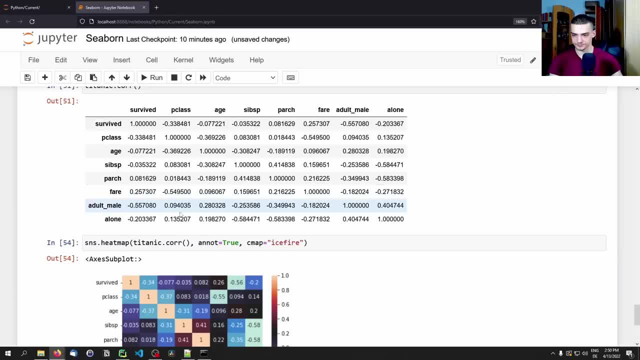 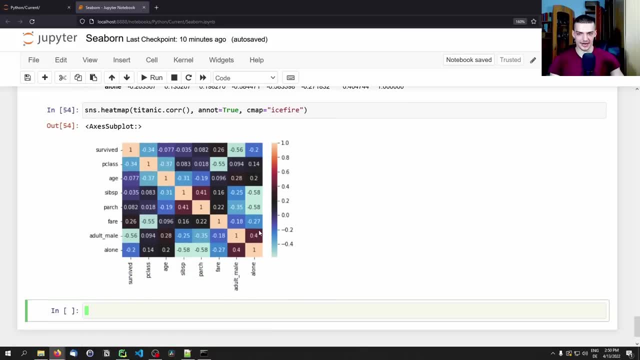 And we also have different color maps, like ice fire or something like that. And yeah, this is one of my favorite plots. This is when I actually use very often. whenever I look into a data set and I want to predict something, I always look. 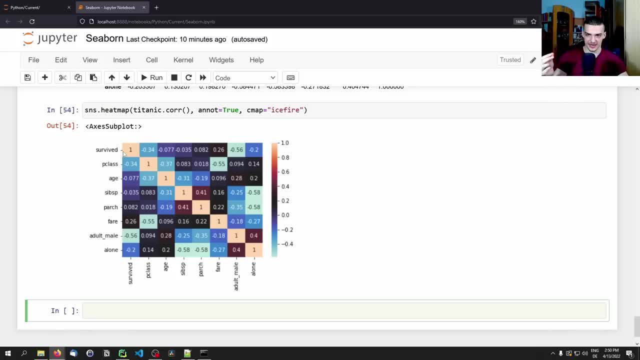 okay, which features are correlated? especially if I want to predict a survival, I want to know which of the features is highly correlated with survival. So here you can see. what is that? Adult male. If you are an adult male, you're probably not going to survive. 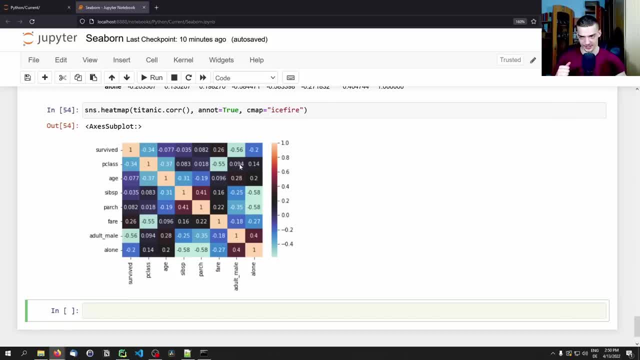 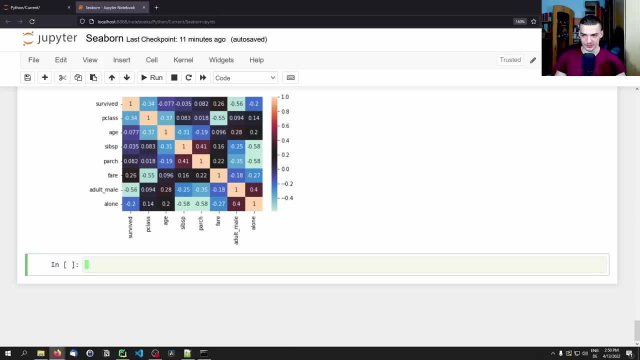 or the probability of you surviving is not very high, as we can see here. Now, last but not least, I want to show you a plot that I'm not actually quite sure I understand, So I don't want to talk too much about how it works here. 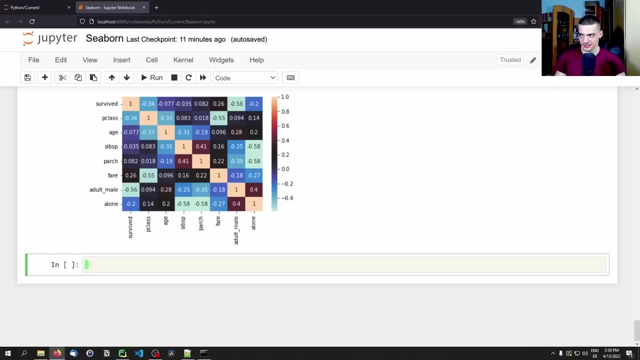 But I want to just show you that plot because it is essentially a dendrogram. It is a cluster map, SNS dot cluster map, And now we can take- I don't know, let's take the iris data set We're going to take. 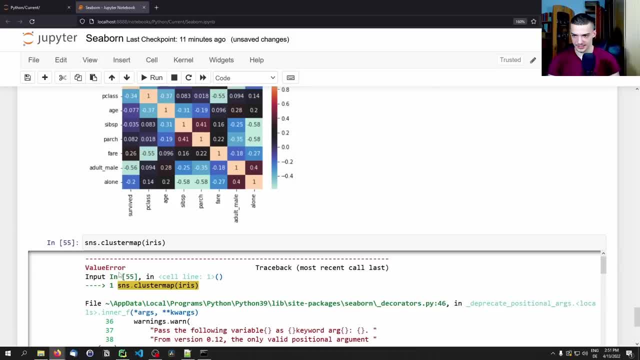 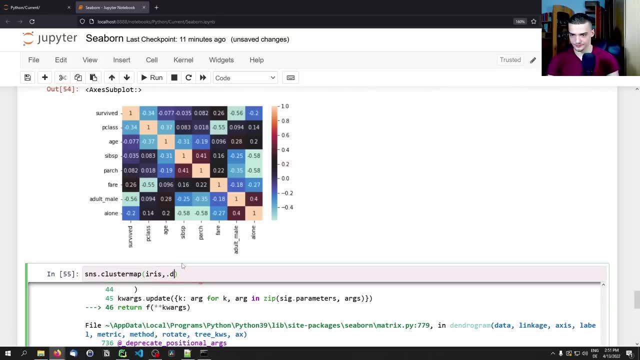 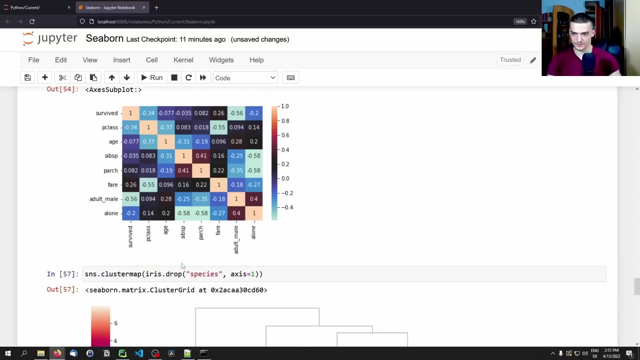 I think we cannot just plot the iris data set. I think we need to drop the features that are not numeric. So the species: we're going to drop the species, axis one, And now we have this cluster map here. Essentially, this is clustering the individual instances. 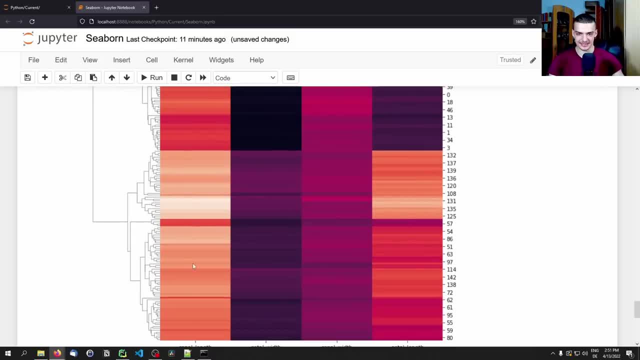 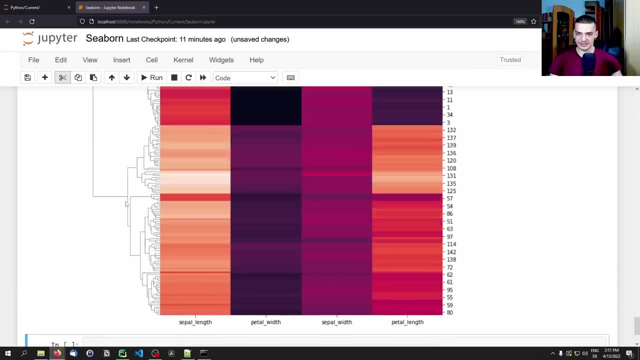 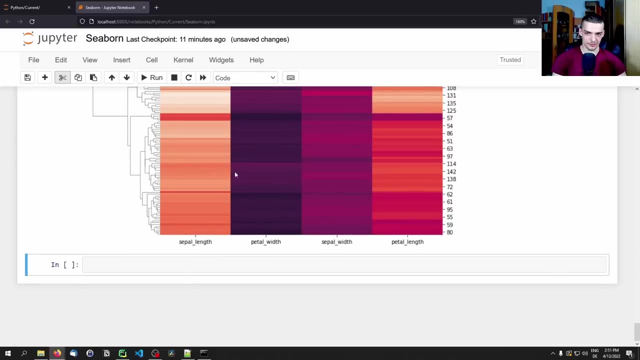 obviously into clusters And this is indicated by colors. Again, don't ask me about any details about this plot, but it can be quite useful if you're dealing with unsupervised learning and if you want to visualize clusters. probably it makes more sense for smaller plots. 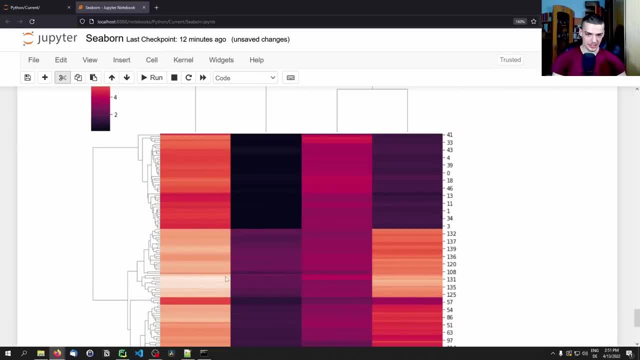 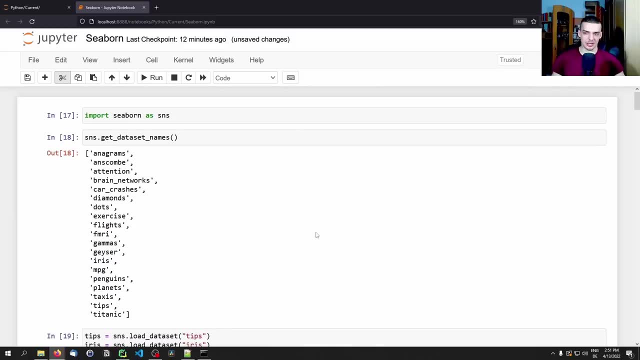 So it doesn't have to look as chaotic as that, But the individual colors here are representing clusters, So those are definitely not all the plot types that you can find in Seaboard. I recommend you check out the documentation. There are a lot of interesting and more advanced examples.